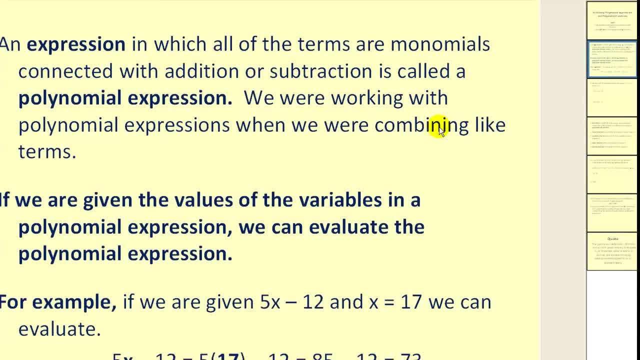 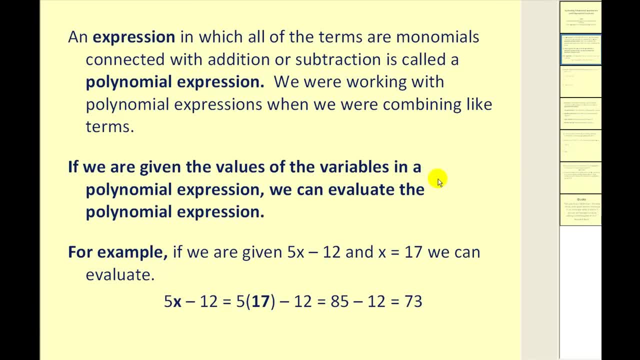 We were working with polynomial expressions when we were combining like terms in the previous video. If we are given the values of the variables in a polynomial expression, we can evaluate the polynomial expression. So, for example, if we have the expression 5x minus 12, 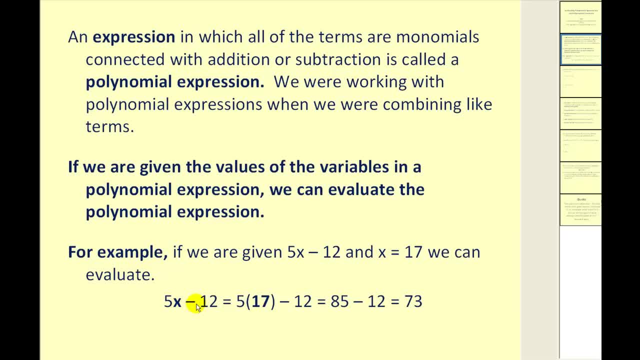 and x equals 17,. we can replace x with 17,. this is called substitution, and then evaluate the expression. So, instead of 5x minus 12,, we have 5 times 17 minus 12, which equals 73.. Let's try a couple of our own. 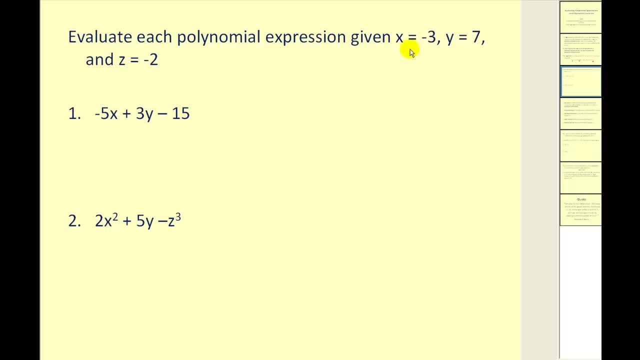 We want to evaluate the polynomial expression. We would have to write these expressions given: x equals negative 3,, y equals 7, and z equals negative 2.. So we would have, instead of negative 5 times x, we'd have negative 5 times negative 3,. 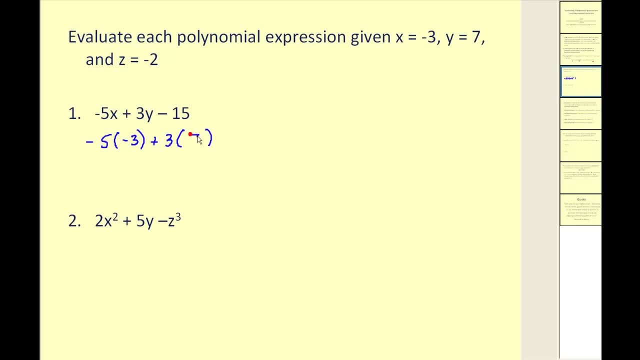 plus instead of 3 times y, we'd have 3 times 7 minus 15.. Now we simplify this expression to get 15 plus 21 minus 15, which is equal to 21.. Now we can easily check these with the use of the graphing calculator. 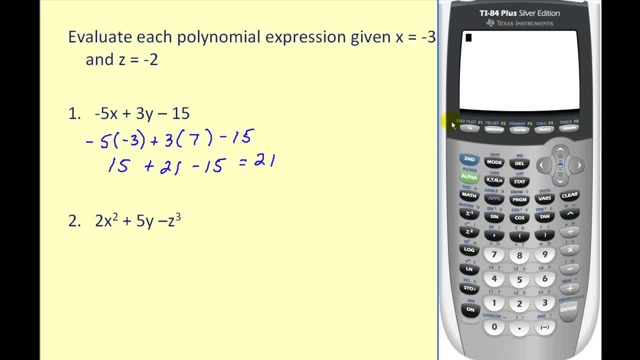 let me show you that The first thing we have to do is store the values into the variables. So in order to store negative 3 in for x, we press negative 3, store x. enter Y is equal to 7,. 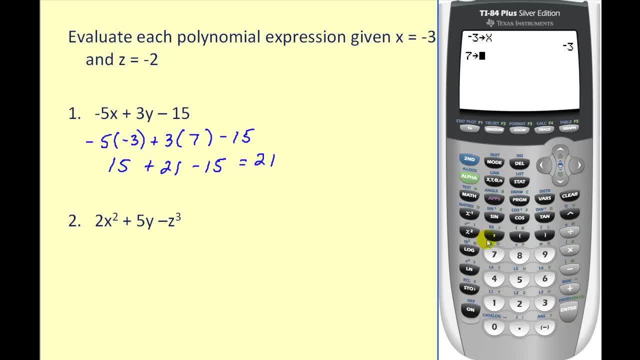 so we press 7 store. Now to access the y, we hit alpha 1, enter and z equals 7.. is equal to negative 2, so we press negative 2, store. alpha 2 will give us z. press enter. 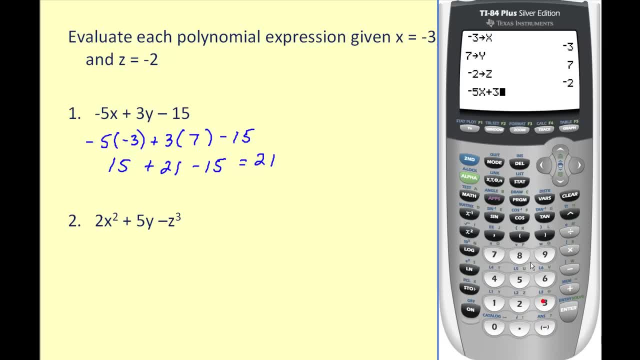 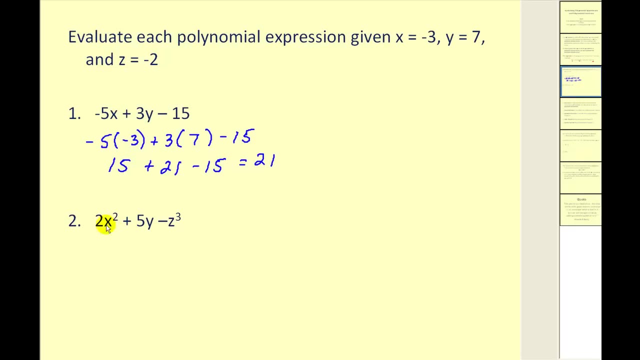 Now we can just type in the given expression negative 5x plus 3y minus 15 to verify our answer. Okay, let's try another Again. the first step is to replace the variables with the given values. So here we have, instead of 2 times x squared, we have 2 times negative. 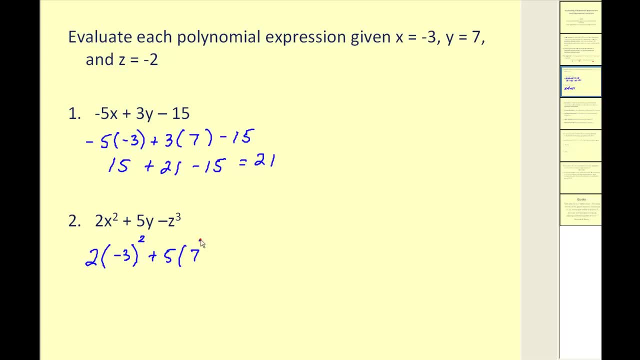 3 squared plus 5 times y, but y is 7, minus z, but z is equal to negative 2.. Let's simplify our exponents first: Negative 3 squared would equal 9,. negative 2 cubed would equal negative. 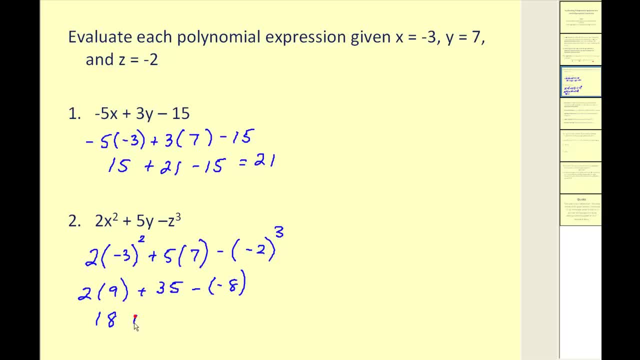 8.. Let's continue to simplify Here. we'd have 18 plus 35, negative 3 squared would equal negative 8.. Let's continue to simplify Here. we'd have 18 plus 35, negative 3 squared would equal negative 8, plus 8,, which is equal to 61.. Again, let's verify this with the. 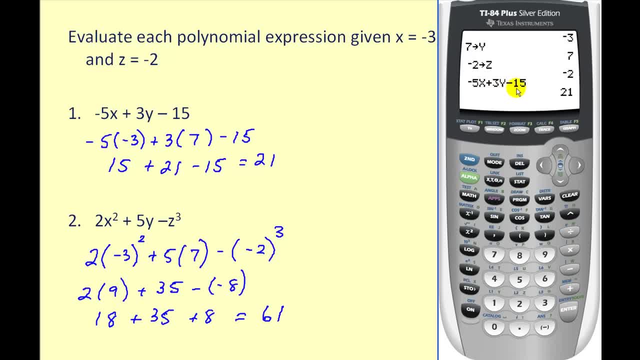 graphing calculator. Since we already have the values stored for the variables, we can just enter in the expression 2x squared plus 5y minus z to the third power, and that checks our work. Okay, now let's talk about polynomial functions, A function in which all of our 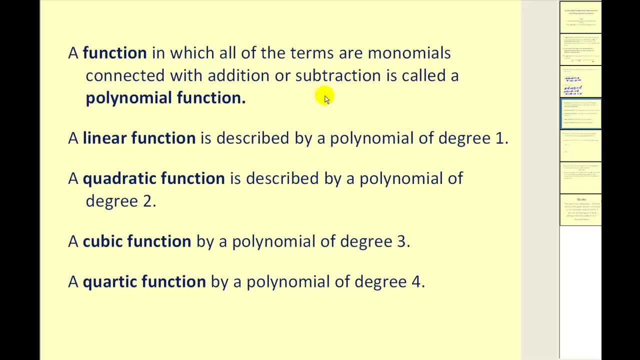 terms are monomials connected with addition or subtraction is called a polynomial function. A linear function is described by a polynomial of degree 1.. A quadratic function is described by a polynomial of degree 2, a cubic degree 3, and a quartic degree 4.. So here we have. 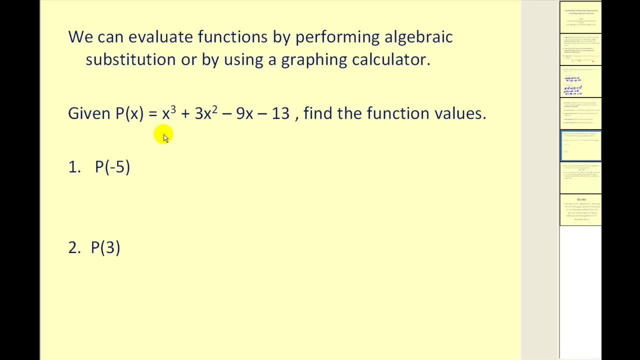 a polynomial function of degree 3, and we're asked to find the function values. and we're asked to find the function values. So it's essentially the same as evaluating an expression, except the notation is different. Here we have a function where before we just had the 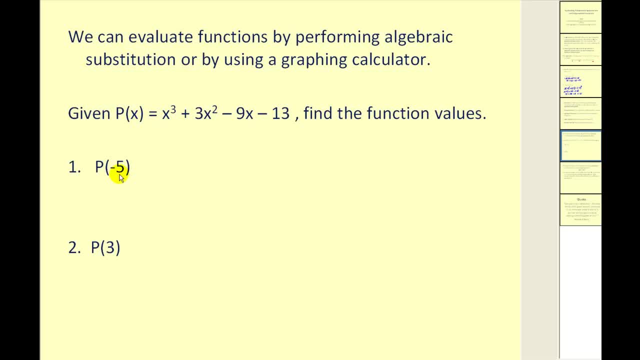 expression. Here we can see the x has been replaced with negative 5, and this is exactly how we evaluate this function when x is equal to negative 5, by performing substitution. So we have negative 5 cubed plus 3 times negative 5 squared minus 9 times negative 5 minus 9,. 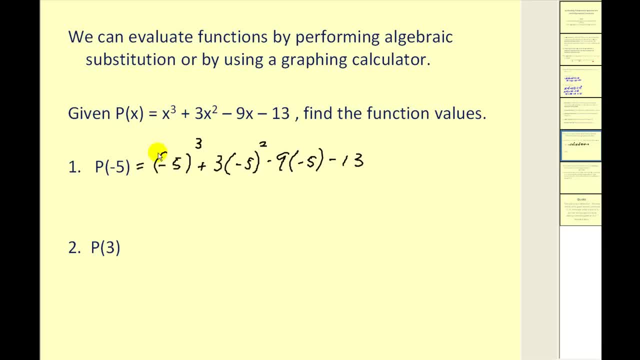 minus 13.. So now we need to simplify this. Negative 5 cubed would equal negative 125.. Negative 5 squared would equal positive 25 times 3,, that would be 75.. Negative 9 times negative 5 would be plus 45, and then minus 13.. We simplify all of this. we should obtain: 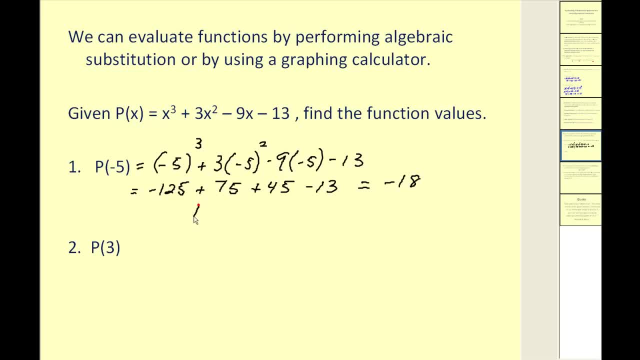 negative 18.. So, in conclusion, p of negative five is equal to negative eighteen. Now I want to make the connection that this actually represents a point on this function, and that point would be: when x is equal to negative five, y would equal negative eighteen. 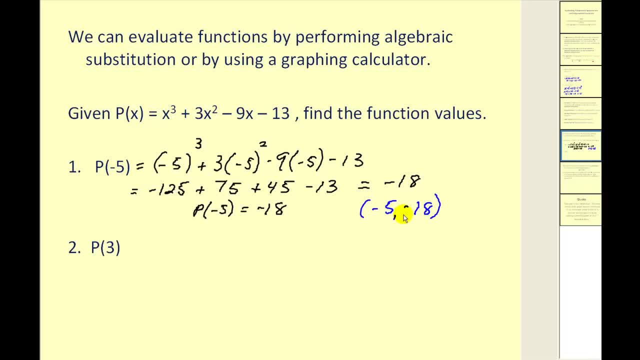 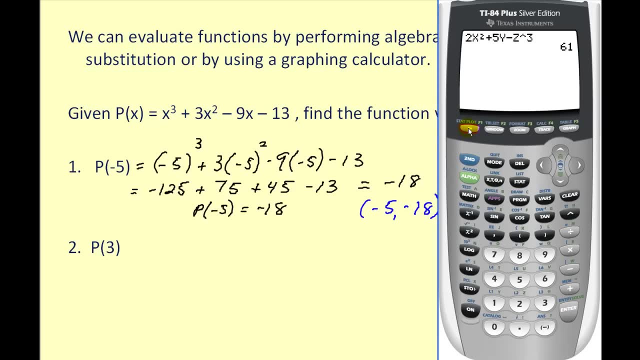 So if we graph this function, this point would be on the graph. Now again, let's verify this on the graphing calculator. Now we could do it the same way. we did the expression, but since it is a function in one variable, let's go ahead and type it into y1, and let's utilize the table function. 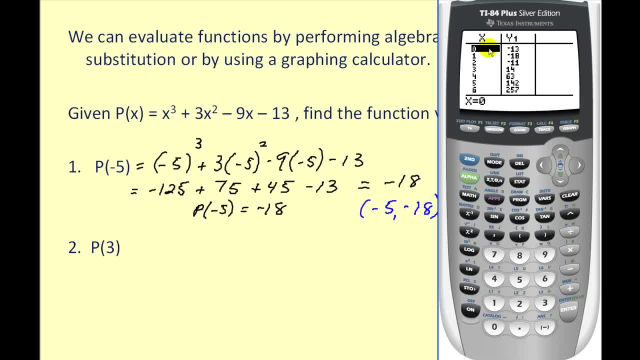 this time. So if we press second graph, my table is set on the automatic feature so I can just scroll up to negative five and see that negative eighteen is the value of the function when x is negative five. so that verifies our answer. 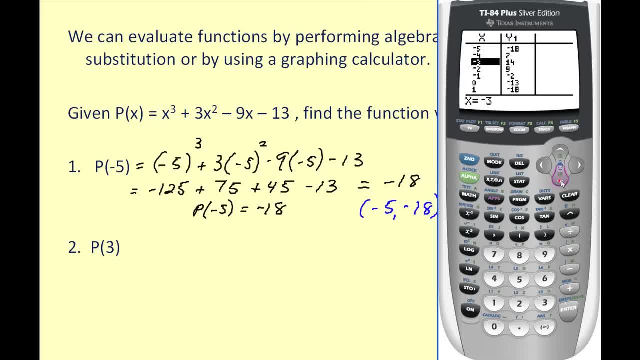 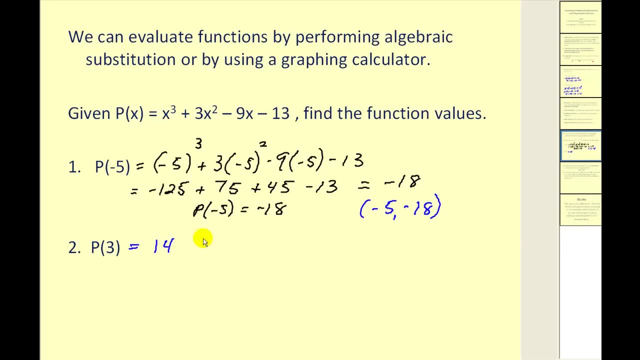 And in fact, if we wanted to take the shortcut for number two, we could scroll down to x equals three And see that when x is equal to three, y is equal to fourteen. therefore, p of three is equal to fourteen. Now I would encourage you to verify this by hand, as we did on number one, but to save 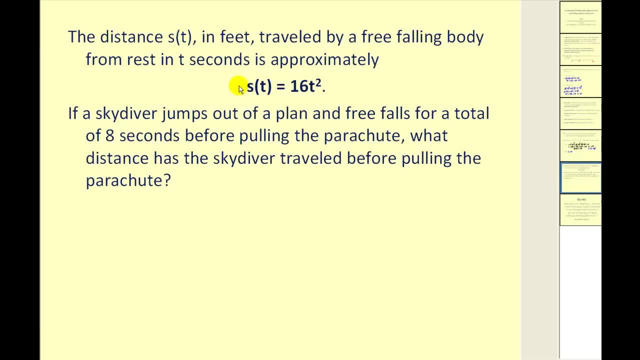 time, I'm going to go ahead and go on to the next problem. Here's an application of a degree two polynomial function, better known as a quadratic function. It states that distance s of t in feet traveled by a function is equal to the distance s of 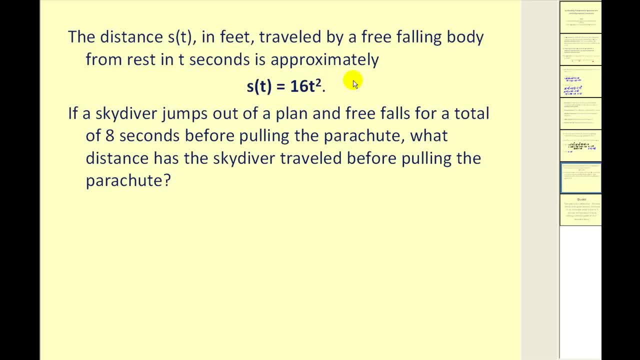 t in feet, traveled by a function. If a skydiver jumps out of a plane and free falls for a total of eight seconds before pulling the parachute, what distance has the skydiver traveled before pulling the parachute? We're given the time of eight seconds, so we need to find s of eight, which is equal. 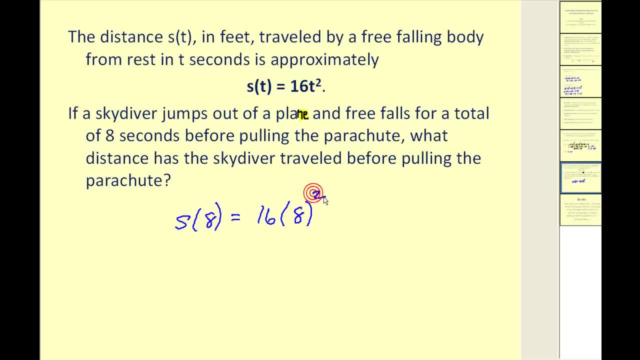 to sixteen times t squared. but now we know t is eight, So this would equal sixteen times sixty-four, which is equal to one thousand twenty-four, And the units for s of t is in feet, so the skydiver has fallen one thousand twenty-four.